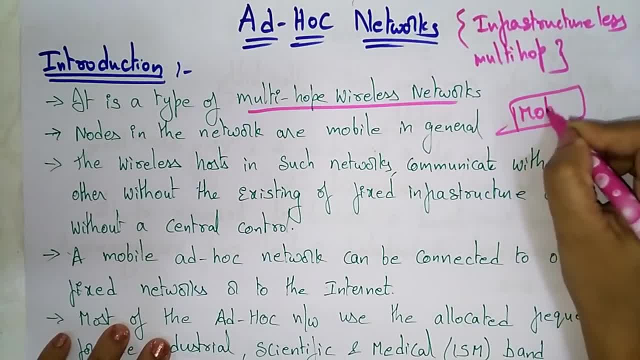 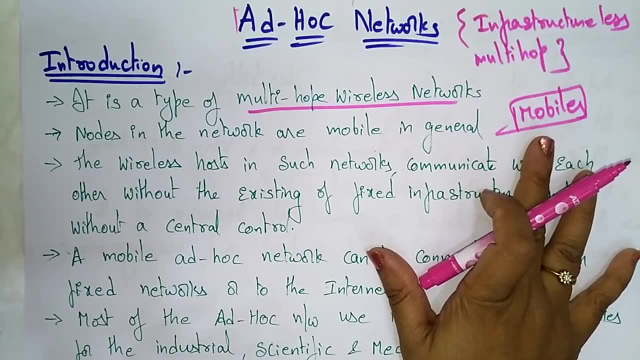 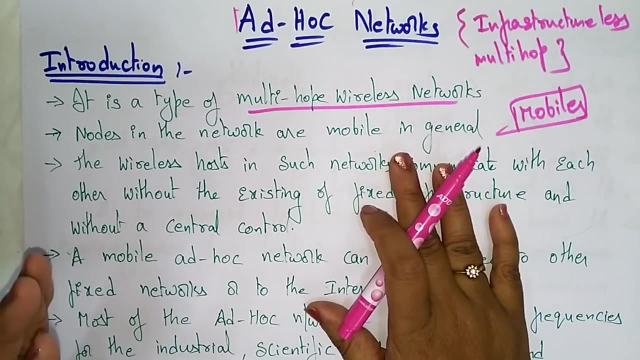 So the ad-hoc networks will be work on mobiles Mainly. we establish these ad-hoc networks in the mobiles. in the case of mobiles, If you want to communicate directly with the mobile, from mobile to mobile, you can go for ad-hoc networks. Okay, so which is an infrastructure? less If it is a single. 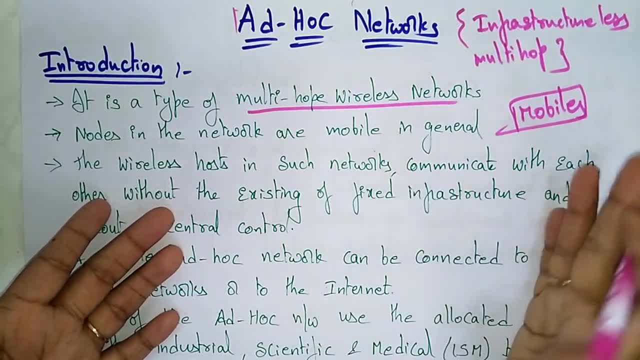 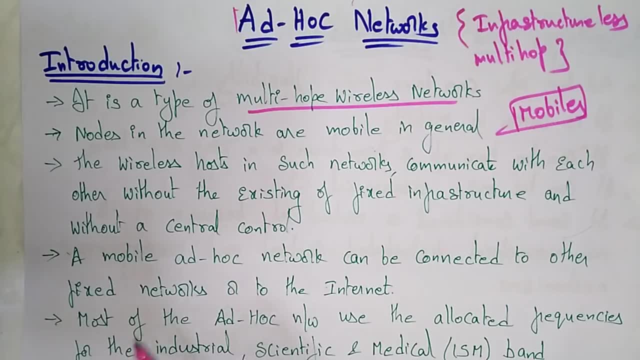 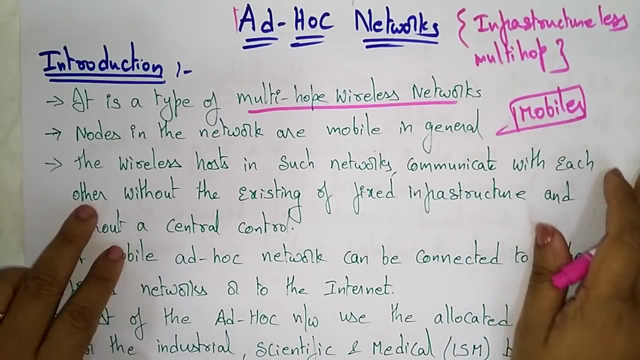 hope you can go for directly bluetooth From mobile to mobile communication. you can directly go for the bluetooth if a single hope, If it is a multi-hope, you you have to work on ad-hoc networks. The wireless host in sash networks communicate with each with each other without the existing of fixed infrastructure and without a 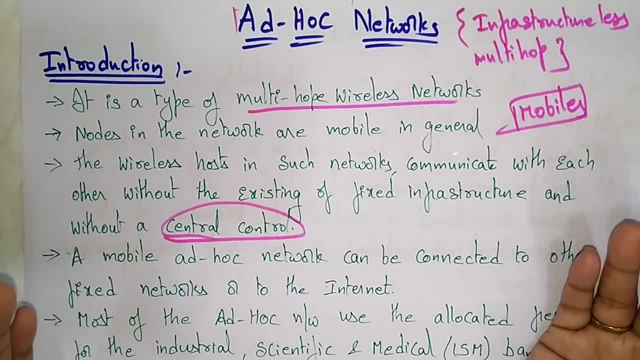 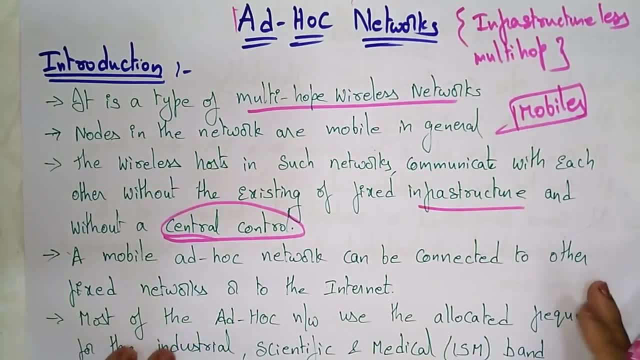 central controller. So there is no need of central controller here. So just if you want to communicate from one mobile to another mobile, you can directly communicate. There is no need of infrastructure. Okay, a mobile ad-hoc networks can be connected to other fixed networks. 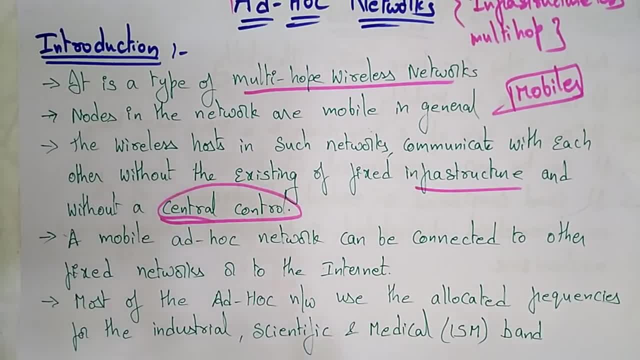 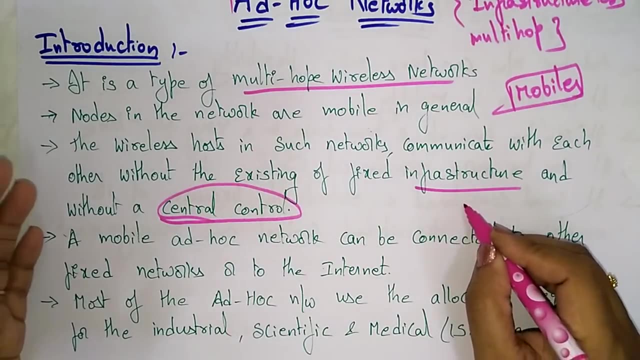 or to the internet. So this is a thing you have to. So, whatever the mobile device that you have to be connected- that should be internet connection- will be there. Okay, so that is another thing you can call it as a. that is the infrastructure. Okay, so this is, this is the router Let us take. this is the. 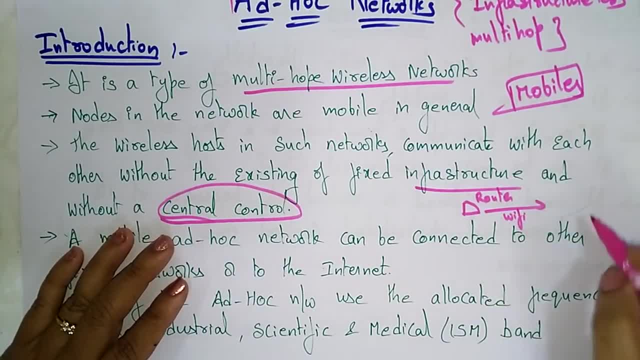 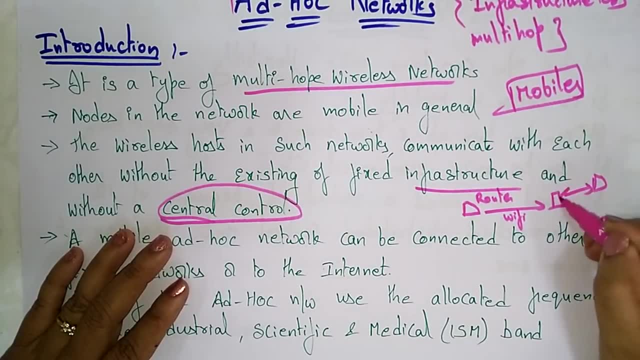 router which you are getting the Wi-Fi signals, Wi-Fi signals. So here, one device is there, another device is there and the device is there. So if you want to communicate these two devices, then you can directly communicate. We are talking about only this part, So a mobile ad-hoc network can be. 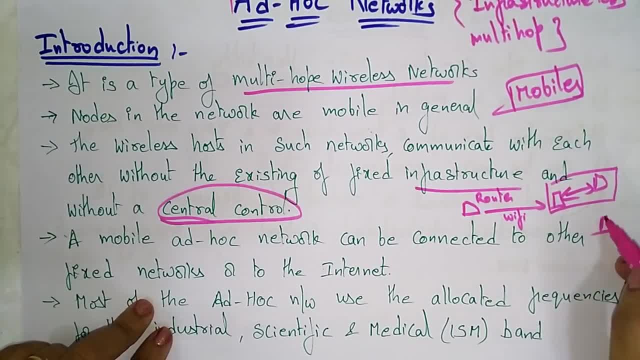 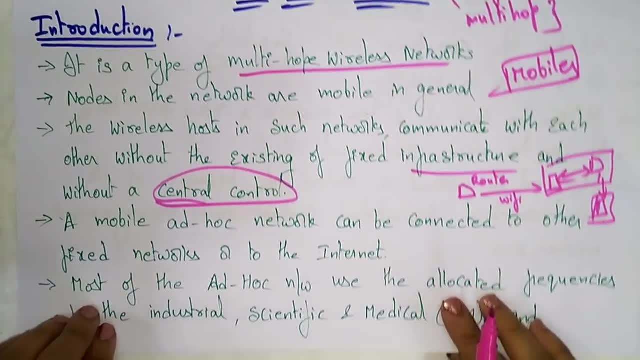 connected. This is a mobile ad-hoc network. This is a mobile ad-hoc network and here the computer is a mobile ad-hoc network, So these can be connected to a fixed network or to the internet. Most of the ad-hoc networks use the allocated frequencies for the industrial, scientific and 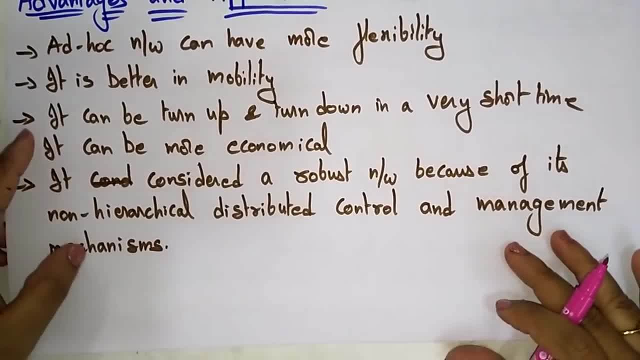 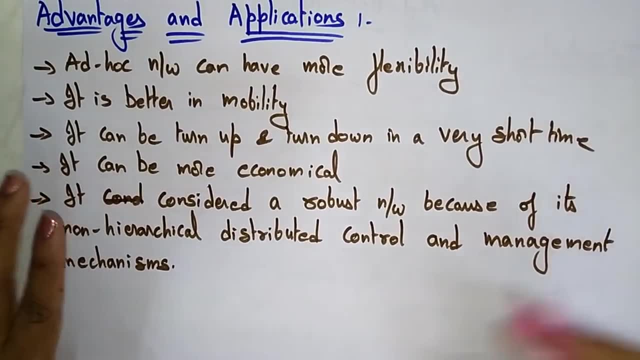 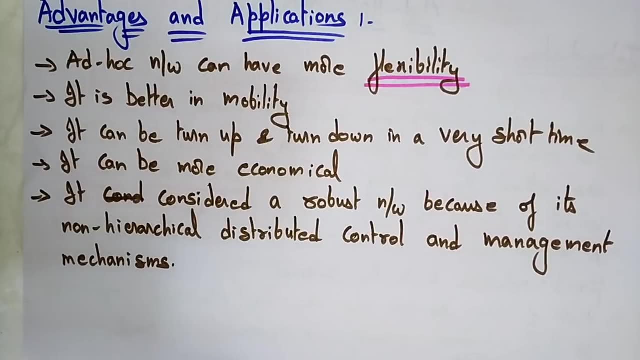 medical banks. Now let's see some of the advantages and applications of these ad-hoc networks. So the advantages of this ad-hoc networks is ad-hoc network can have more flexibility. it is have more flexibility. Why ad-hoc networks are more flexibility? because they are temporary devices. ad-hoc networks are 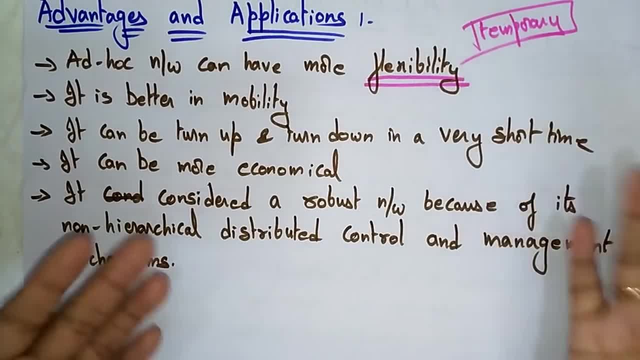 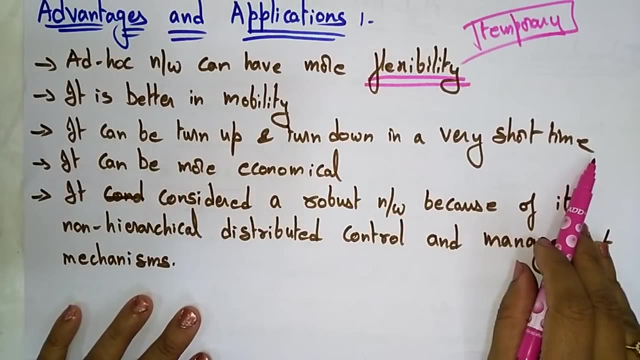 temporary. Okay, if you want you can add. if you want you can delete. Okay, so it is a better in mobility. So just there is an access of placing and removing. It is a better mobility. It can be turn up and turn down a very short time. it can be more economical. it considered a robust network. 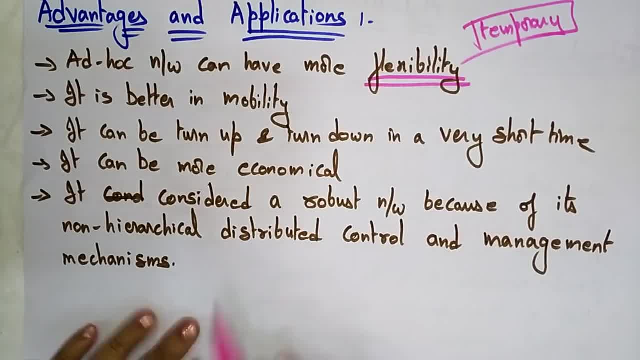 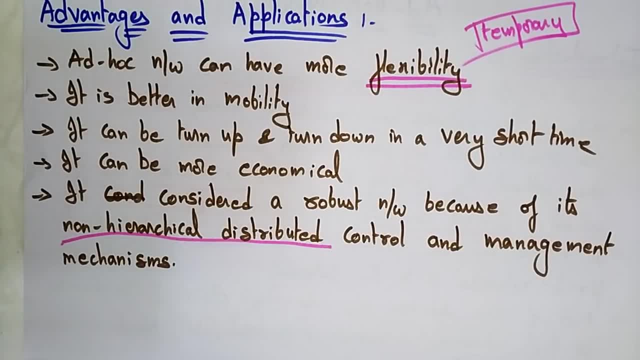 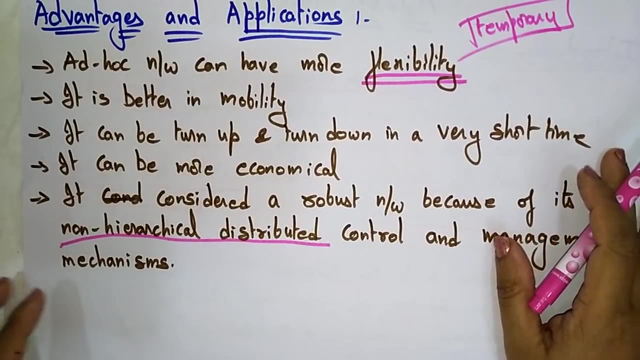 because of its non-hierarchical distributed control and management mechanism. so it can be a robust network because of non-hierarchical distribution, control and management mechanisms. these are the advantages. i think you get one doubt here. i said: ad-hoc networks are the infrastructure, less networks. so i am talking about the 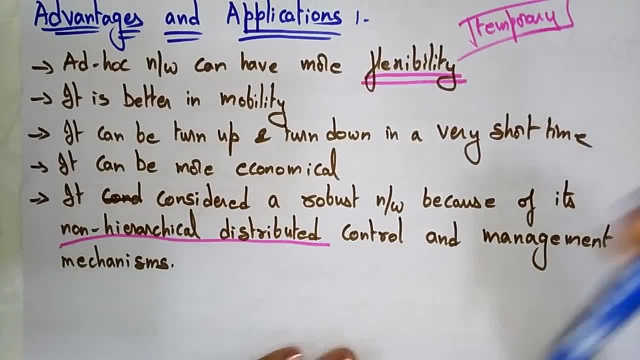 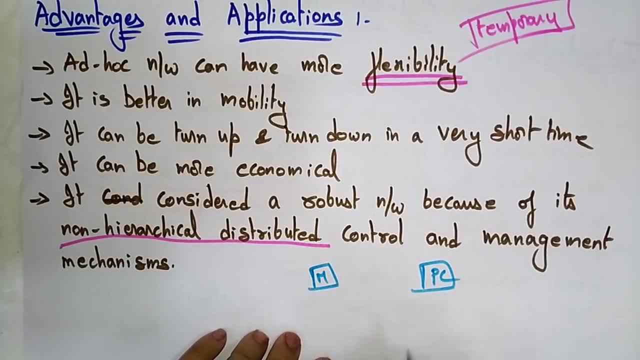 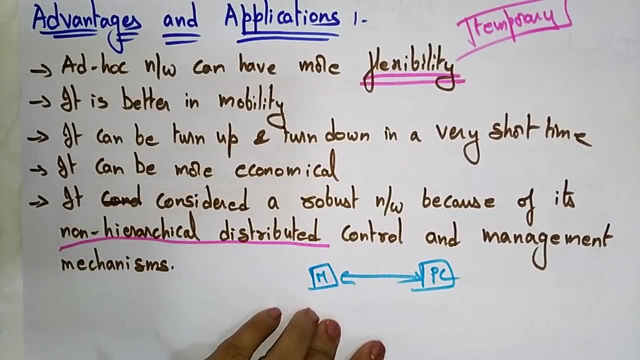 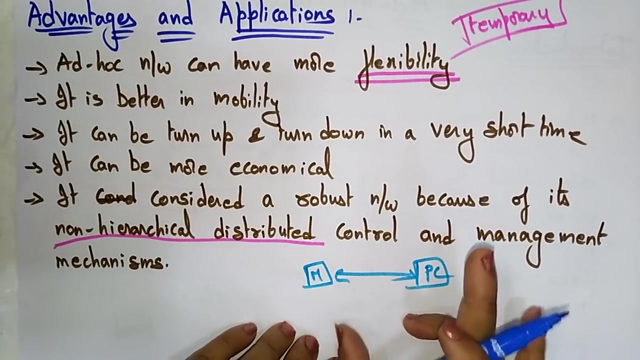 infrastructure, less network, suppose. if i want to communicate, here the mobile phone is there and here the laptop is there, a pc is there. if these two device wants to communicate, how the ad-hoc network will be established in between these two devices. there is already internet connection. is there then ad-hoc? how it will be established? it's very simple. 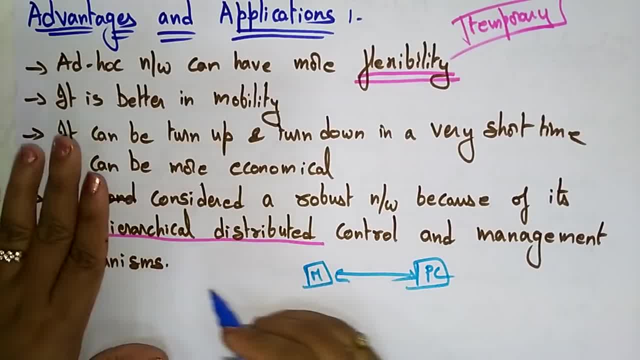 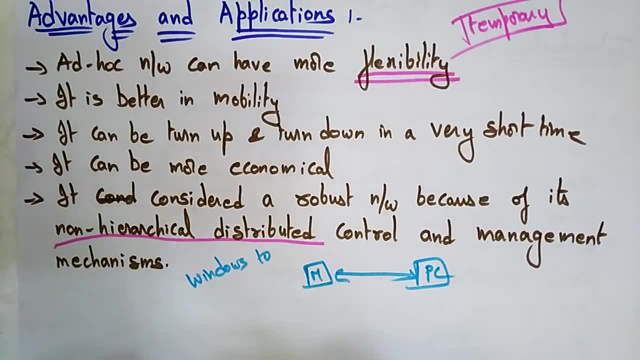 in the previous versions of windows it is very easy. but for if you take for windows 10 operating system, in the command prompt you need to type the commands and you have to be activate the ad-hoc network. whenever you don't require, you deactivate the ad hoc network. 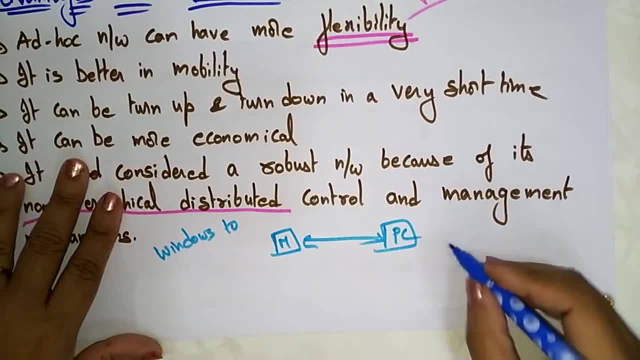 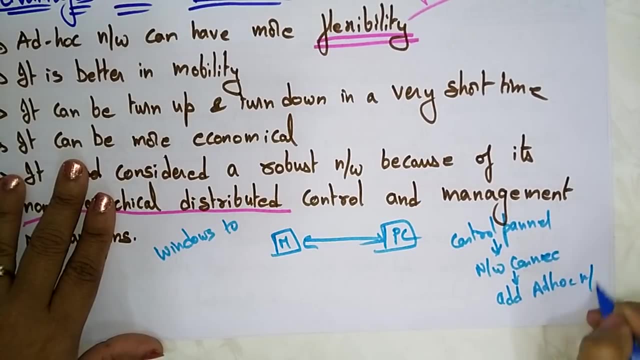 in the command prompt previously, what they are doing? just, you're going to the control panel. in the control panel, control panel, you are going for the network connections and there, in the network connections, you can add the ad hoc network there. so whenever you required, so whenever this is active in your 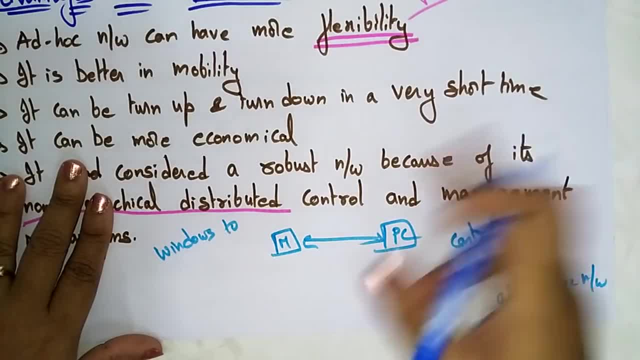 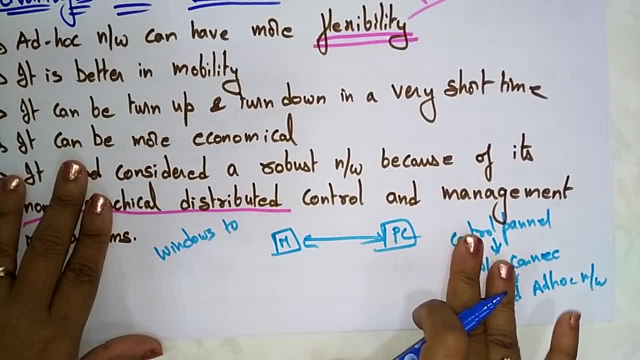 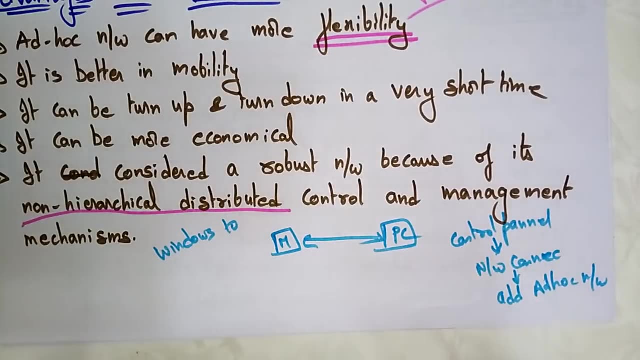 system, you can access the nearby devices, you can directly access the new nearby devices and you can directly communicate the two devices. okay, so that is. in that way you can configure the ad hoc networks, so there is no particular device is required for your in your system, or